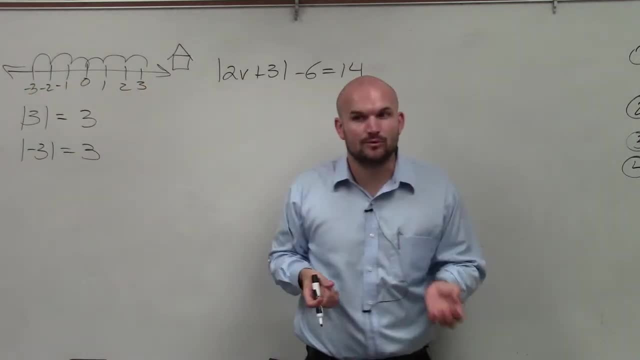 So the important thing you guys remember is the absolute value always equals a positive value. So when I have absolute value of x, let's say 1,, 2,, 3. Let's say it equals 10.. You guys understand that there could be two numbers, that 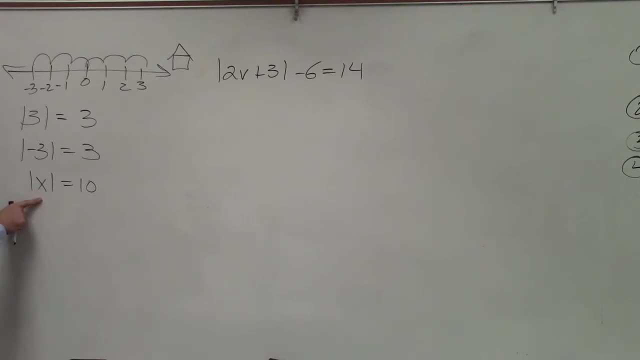 could be in for x. It could be a positive x or it could be a negative x. Does that make sense? There could be two answers. So when we're solving absolute value equations, we're going to be looking for two answers. 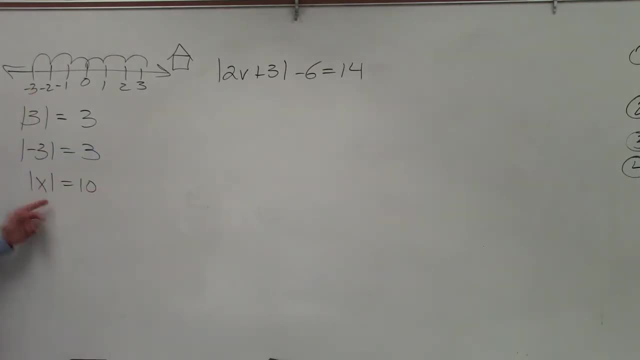 The answer that makes this positive and the answer that's going to make that negative. So when solving an absolute value equation, you guys can see I wrote down the steps over there which I'd highly recommend. The first step is isolate the absolute value. 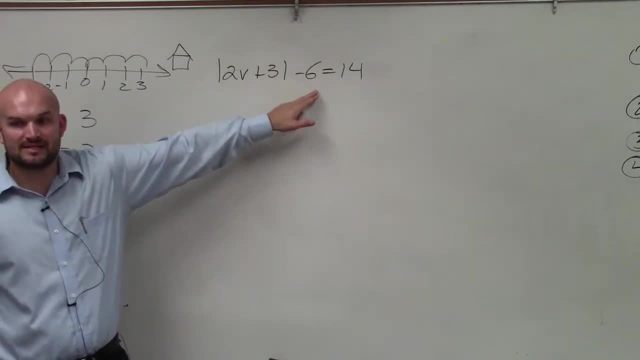 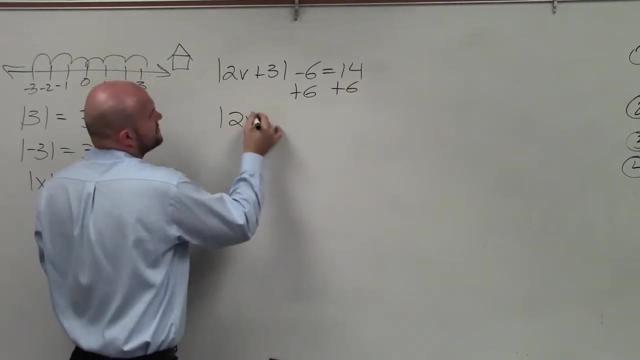 The absolute value sign. Here we can have the absolute value sign as being subtracted by 6.. So we need to undo subtracting by 6 by adding 6.. So I have absolute value of 2v plus 3 equals 20.. 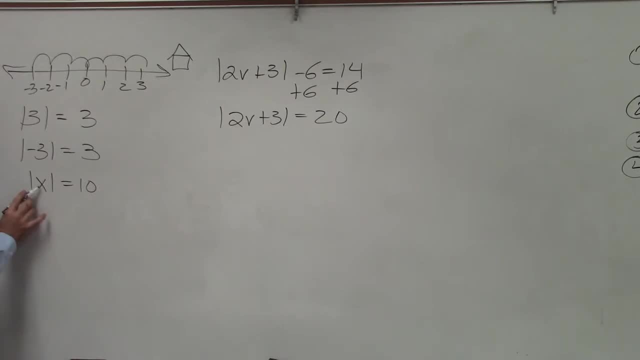 Now the next thing is: remember we said this could be a negative number and a positive number. This could be negative 10, and it could also be 10, or 10. It could be one or the other, But we need to create two cases. 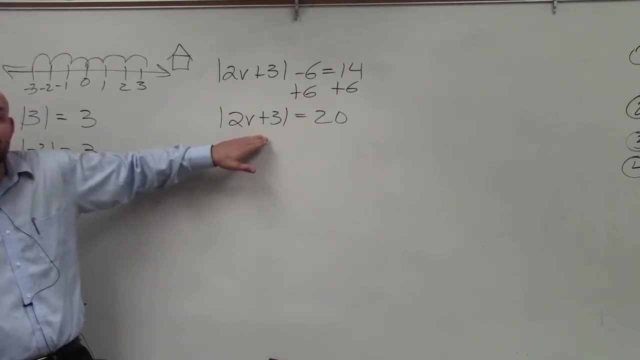 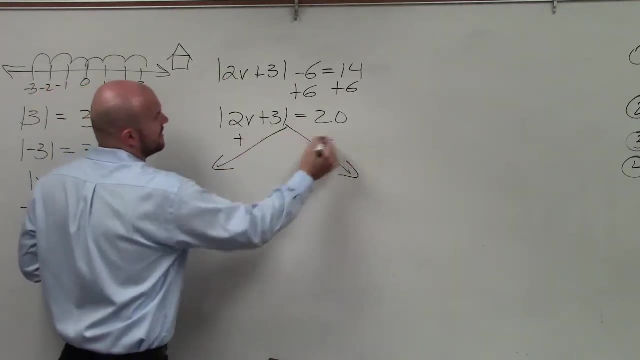 We want to create the case where my variable is positive and the case where my variable is going to make a negative value. So my two cases is the positive and the negative. So you can see I write two cases. So to write the positive case I'm 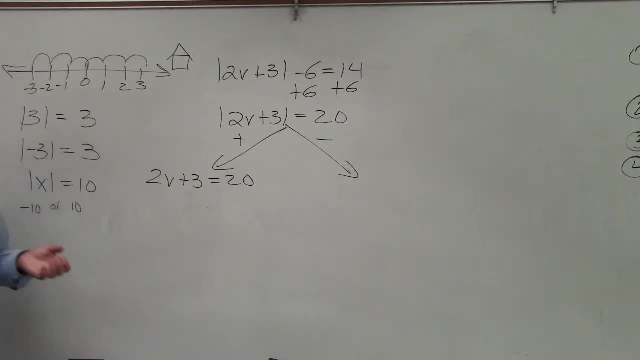 just going to keep the equation exactly as the same. But the important thing is, when you create two cases, you don't need the absolute value sign anymore. Absolute value sign just represents absolute distance from 0. So we create two cases, You don't need that sign. 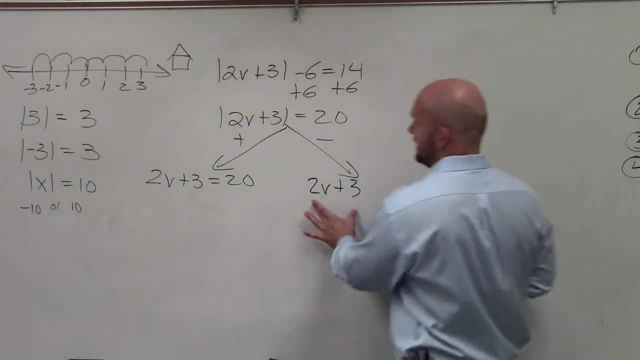 Now to do the negative. all I'm going to do is again write the same thing that was inside the absolute value. But now I'm going to take the negation of the other side. So you're going to negate it. make it the opposite. 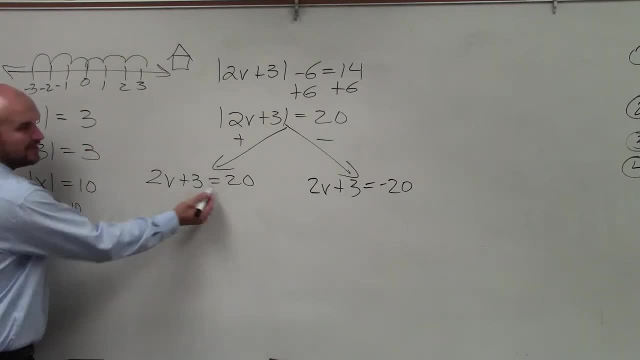 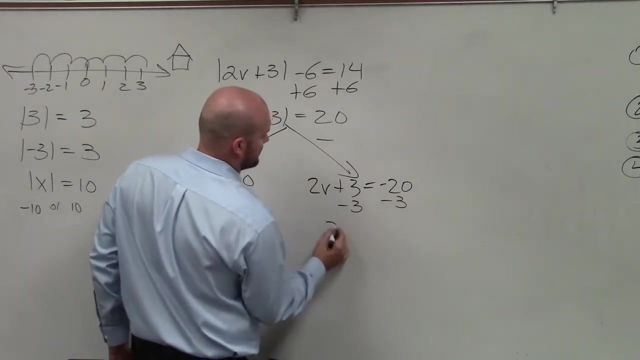 Now step three is just solve. Just like you guys should be happy with this, This is much easier than some of the multi-step problems I gave you. Just solve, And here I'll subtract by 3.. 2v equals negative 20.. 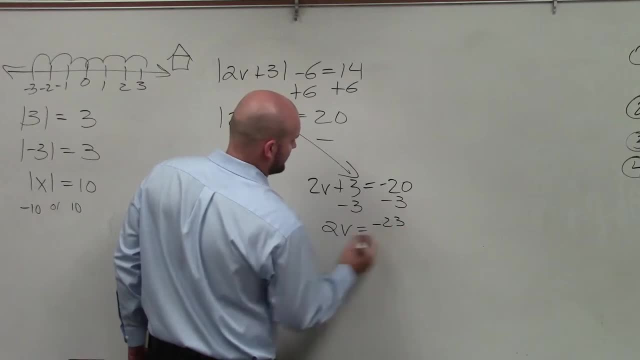 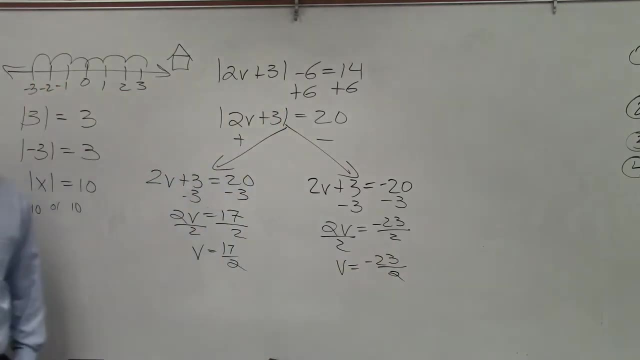 Oh, 17.. Negative 23.. Then divide by 2. Divide by 2. v equals a negative 23 divided by 2.. Not very fun answers, but that's OK. That doesn't mean you did anything wrong. So the last step: now that I've solved, I have two answers. 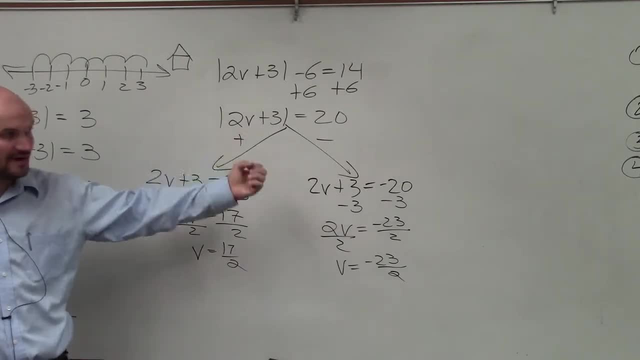 The last step is to check your solutions. This is very, very, very important for absolute value equations, because not always are solutions going to be actual solutions to the equation. So to do that, we have to check the solutions. To check the solutions, what you do is take your values. 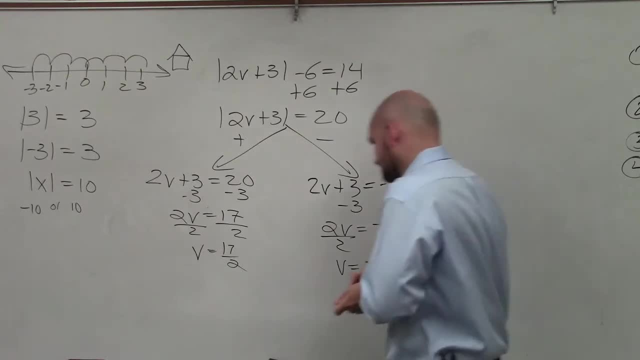 and plug them back into your equation. So you go back to your original equation and I'll write absolute value of 2 times. I'll do the first one: 17 over 2, plus 3 minus 6 equals 14.. 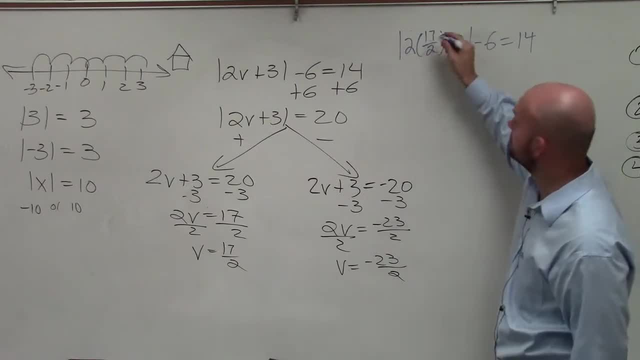 Now I'm just going to do this kind of in my head: 2 times 17 over 2, that's like 2 over 1, right? Yes, No question. So the 2's divide to 1.. So I'm left with 17 plus 3, which is: 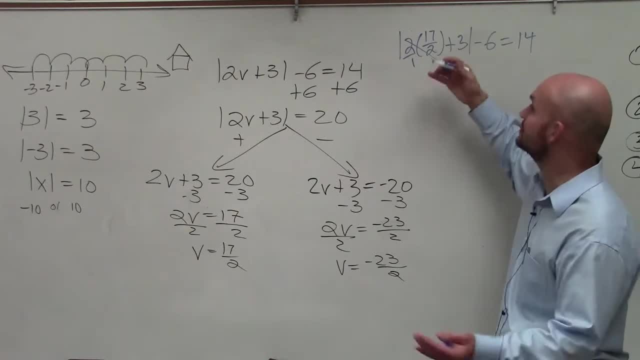 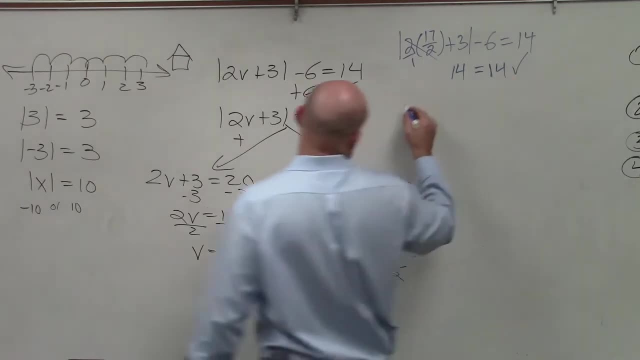 17 plus 3 is 20.. Absolute value of 20 is 20.. 20 minus 6 is 14.. 14,, which is equal to 14,, which is good. Now let's go and check the other solution. 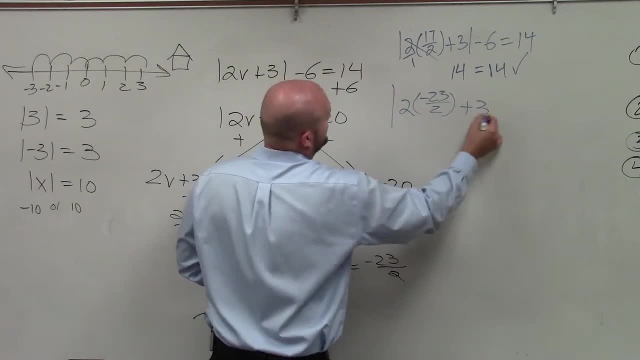 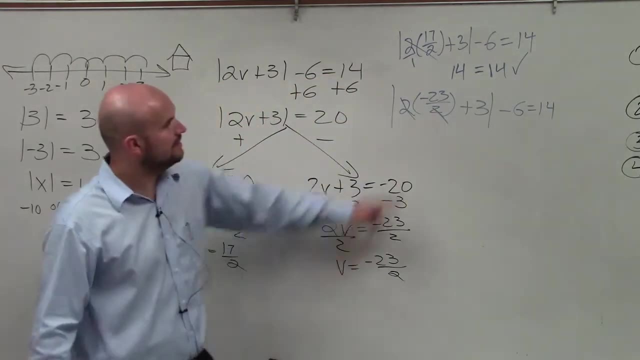 2 times negative. 23 over 2 plus 3 minus 6 equals 14.. So negative 23 over 2, again, the 2's are going to divide to 1. Negative 23 plus 3 is Negative 20. 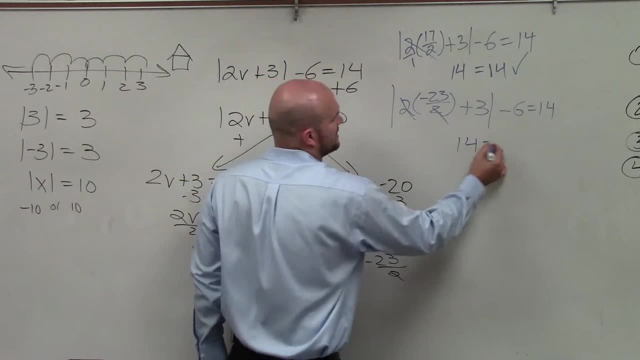 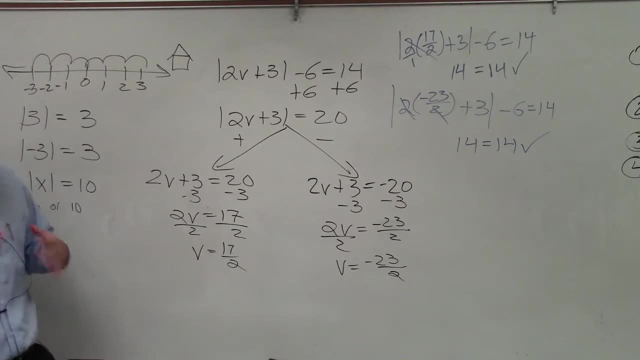 Absolute value of negative 20 is 20.. 20 minus 6 is 14, equals 14.. So in this case, ladies and gentlemen, you have both of your solutions are true, which is nice. However, if you guys might be wondering, 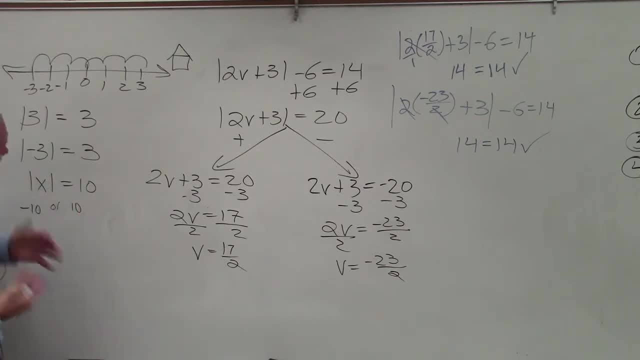 well, why are we checking our work? Both solutions were true. When would be a case where my solution would not be true, where I'd have an extraneous solution? An example: any time when you plug your answer back in, any time you have an absolute value equal to a negative. 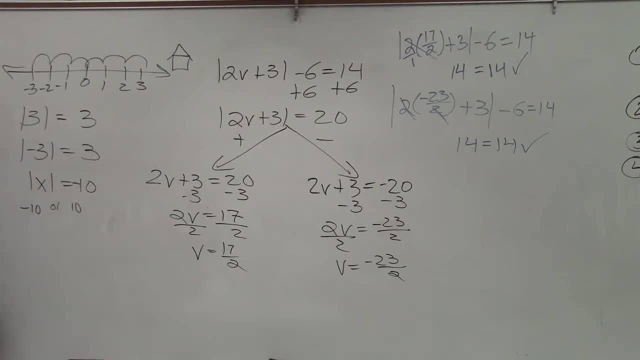 number, you're going to have what we call an extraneous solution or no solution. So any time when you plug your answer back in and you have your absolute value is equal to a negative number, then you're going to have an extraneous solution. 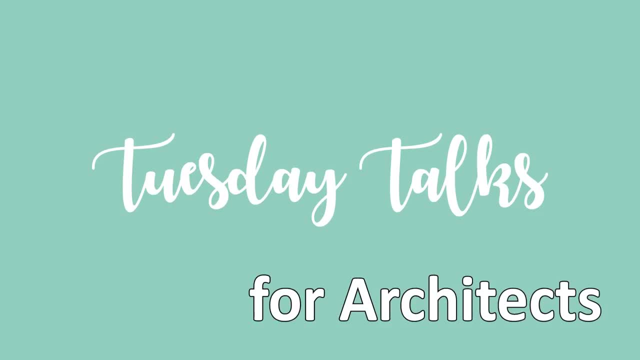 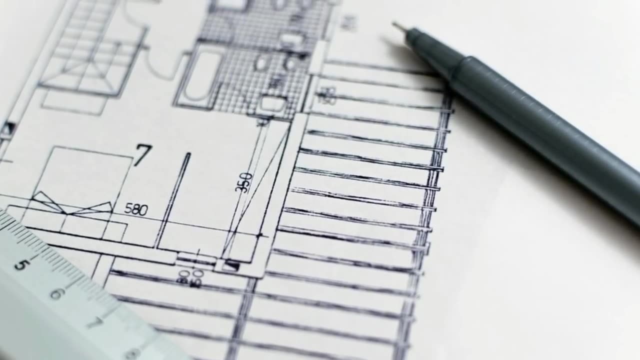 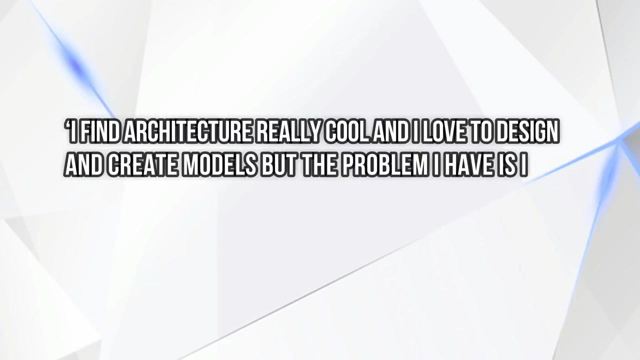 If you ever thought about being an architect but thought you couldn't handle the math, you aren't alone, as you might find this situation a little relatable. I find architecture really cool and I love to design and create models, but the problem I have is I'm weak in maths and physics. 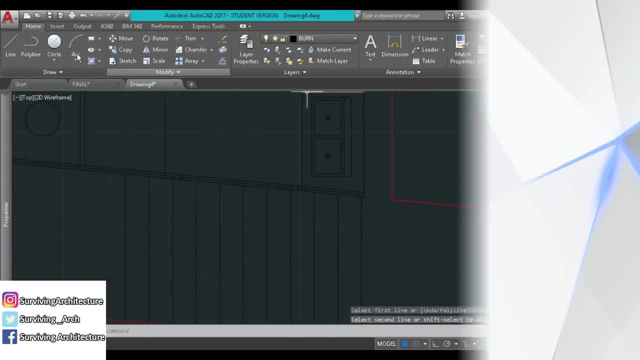 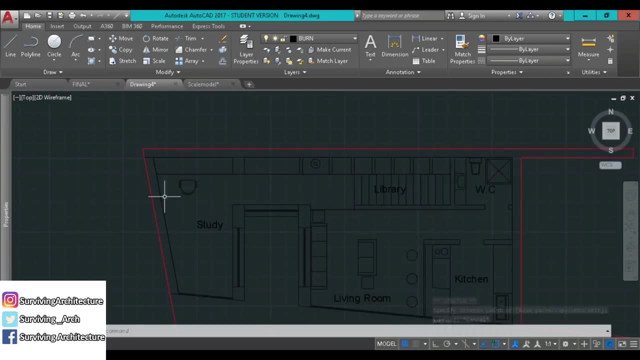 that is why I'm confused whether to go with architecture. It's too bad that more than most people think this, because it's just like a handful of other stereotypes about architects that aren't true. Let me ease your mind by saying you do not have to be great at math to be an architect. 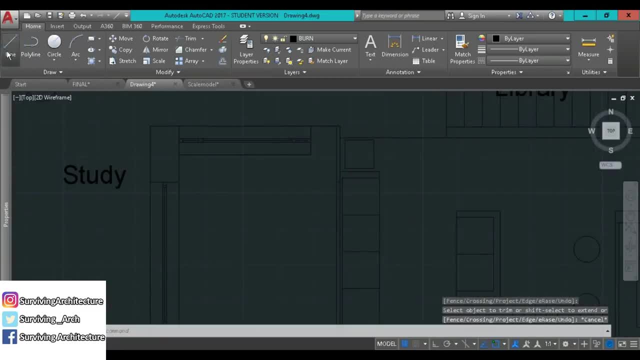 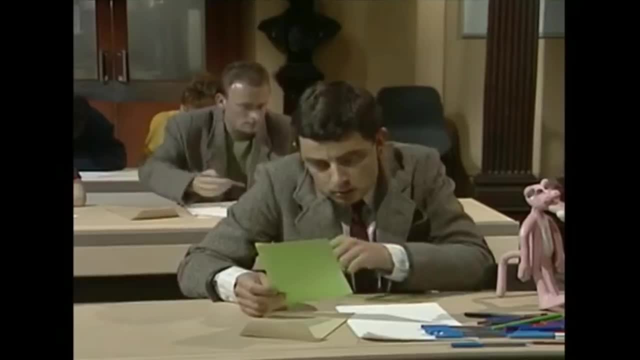 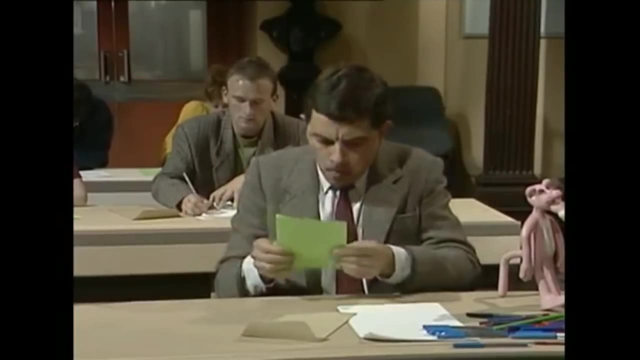 but you can't be completely incapable either. But if you can get through school, then you can get through university too, until you have to do the architectural licensing exam. If you really think being an architect is a good thing, then you're wrong. It's not. 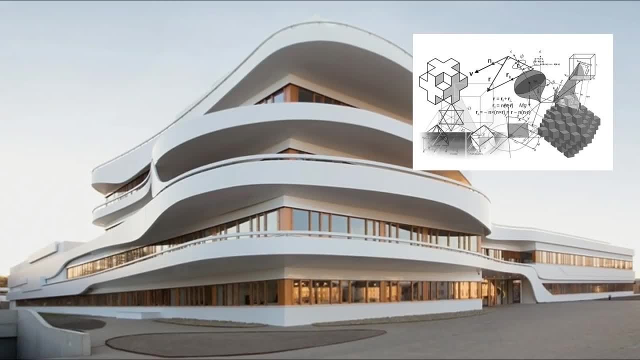 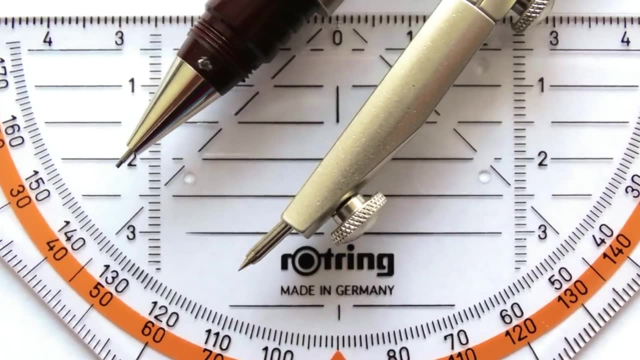 If you think being an architect is the right thing for you, then math shouldn't force you to quit architecture. Math is one of those subjects where many people feel that they either understand it or they don't, and there's some sort of genetic mathematical intelligence.